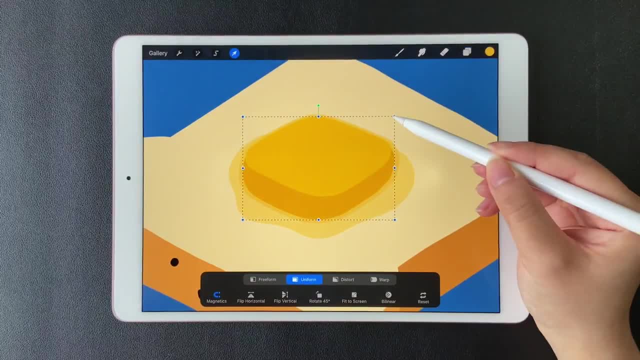 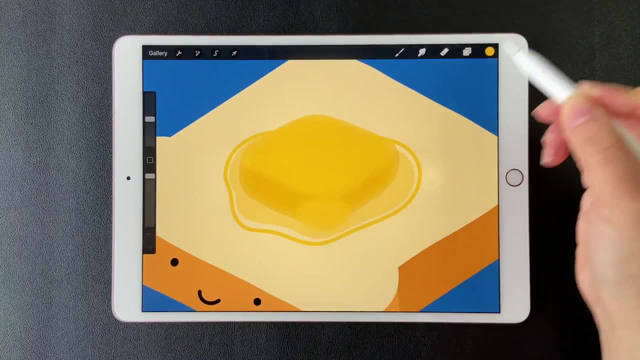 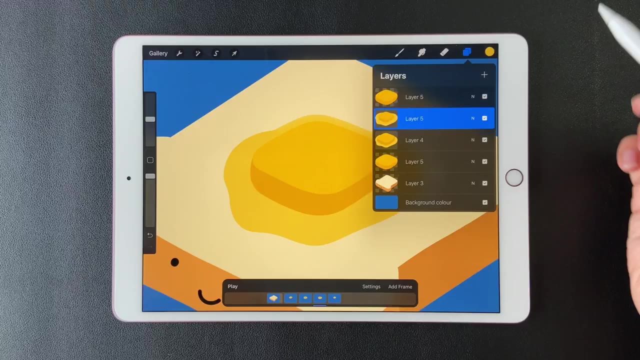 The second frame is done. Select the third butter layer, Make it smaller than the second one. Create a new layer below and draw the melting part which is a little bit bigger than the last one. Duplicate the butter layer for the fourth frame, Merge these two layers and the third frame is finished. 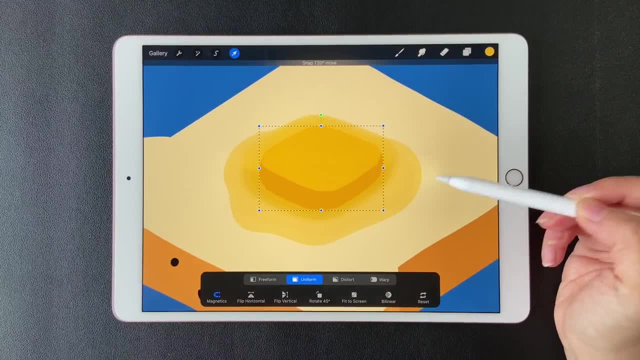 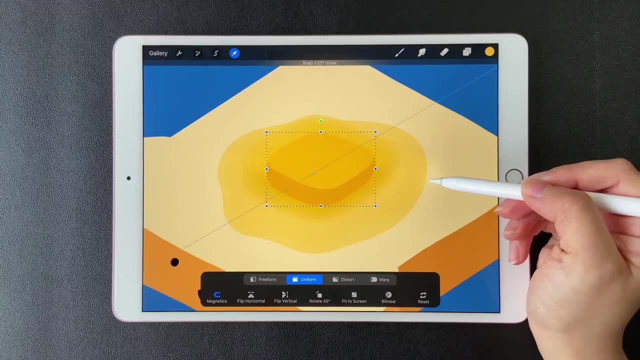 Now you can see the rules For the next frame. reduce the size of the butter. Draw the melting part bigger than the previous frame. Copy the butter layers for the next frame before merging the layers With the onion skin. we can see all the frames with 60% opacity. 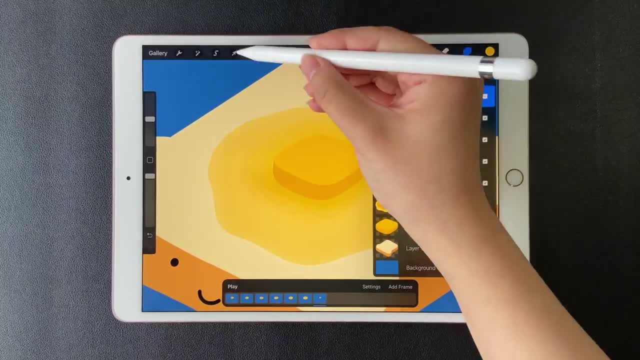 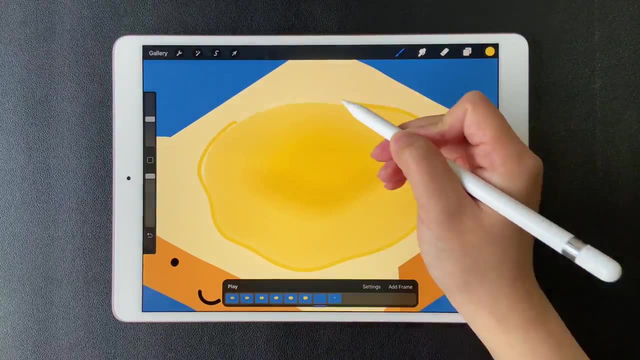 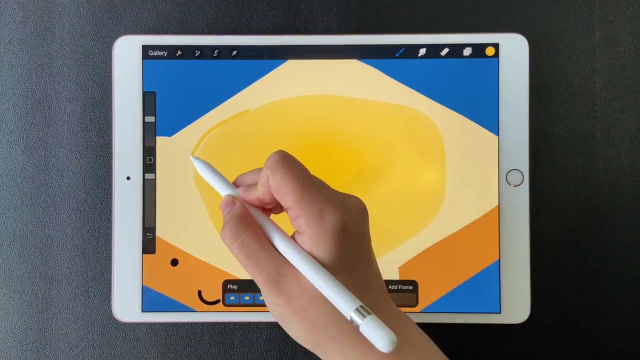 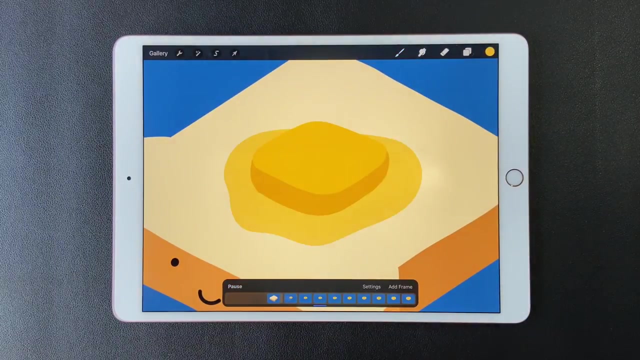 Just keep doing the rest. I'm having 9 frames now For the last layer. just draw the melting part. Now let's hit the play button to check the movements. So it's not hard at all, is it, Since we are working in a digital environment. 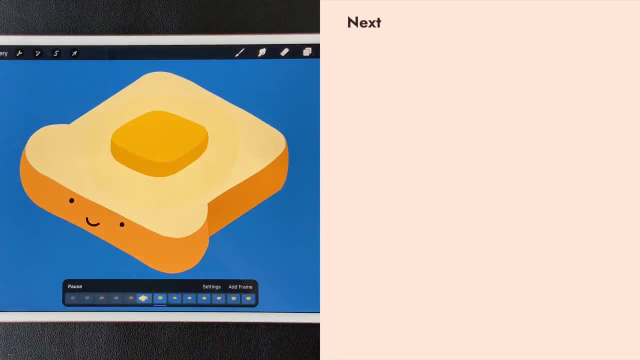 there are some tools in Procreate can help us make animation in different ways and even make the process easier. So stay tuned for the future Procreate animation tutorials. Smash that like button if you have enjoyed this one. Have fun when you create your own piece of animation. And see you next time.